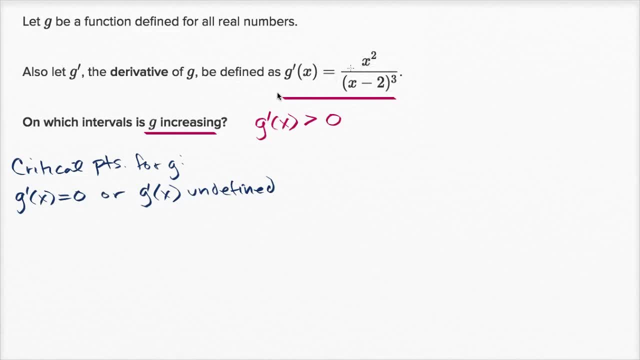 is getting the numerator equal to zero, And that's only going to happen if x, squared, is equal to zero or if x is equal to zero. So that's the only place where g prime of x is equal to zero And where is g prime of x undefined. 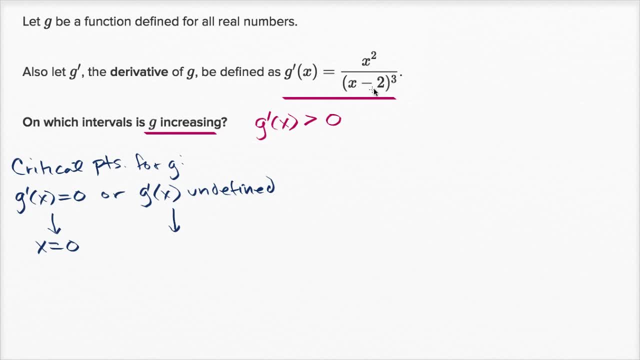 Well, it's going to be undefined if the denominator becomes undefined. The denominator becomes undefined if the denominator is zero, And so that's going to happen. if x minus x is equal to zero, if x minus two is equal to zero, x minus two is equal to zero. 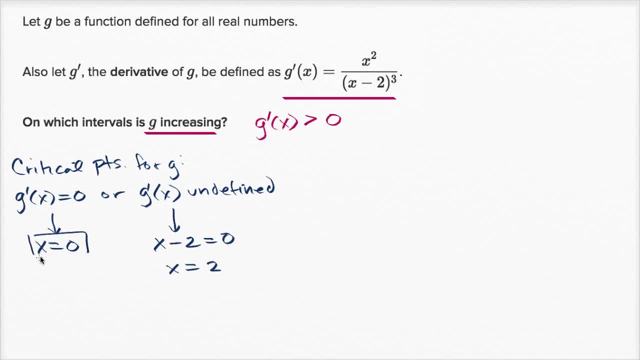 or x is equal to two. So we have two critical points or critical values here, And what I'm gonna do is I'm gonna graph them, let's put them on a number line and let's just think about what g prime is doing. 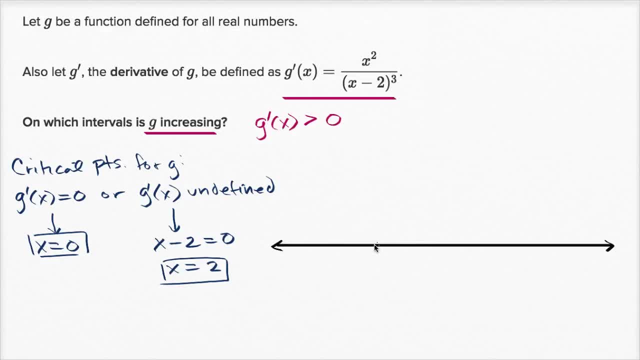 in the intervals between the critical points. So let's start at zero, one, two, three and then let's go to negative one and we have a critical point at. let me do that in magenta we have a critical point at: x equals zero. 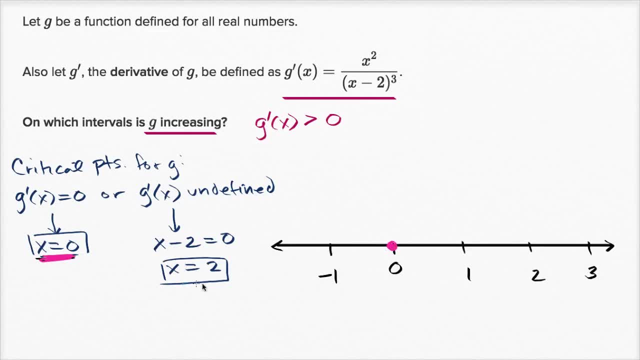 right over there and we have a critical point at x equals two right over there. And so let's think about what g prime is doing in the intervals between the critical values or on either side of the critical values. So let's think about. 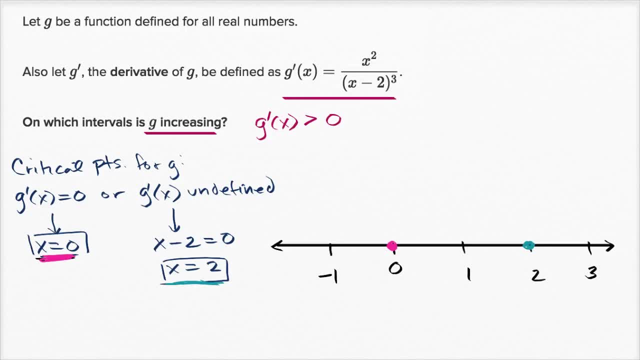 let's first think about this interval. let me do it in this purple color. Let's think about the interval between, between negative infinity and zero. So if we think about this interval, so negative infinity and zero, that open interval. Well, if we look at g prime, 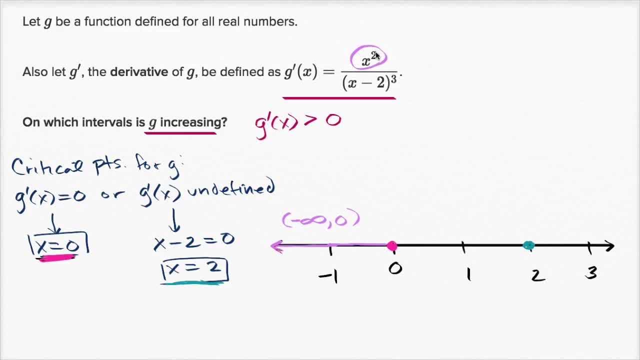 the numerator is still going to be positive. You take any negative value, you square it, you're gonna get a positive value. So this is going to be positive. Now what about the denominator? You take a negative number, you subtract two from it. 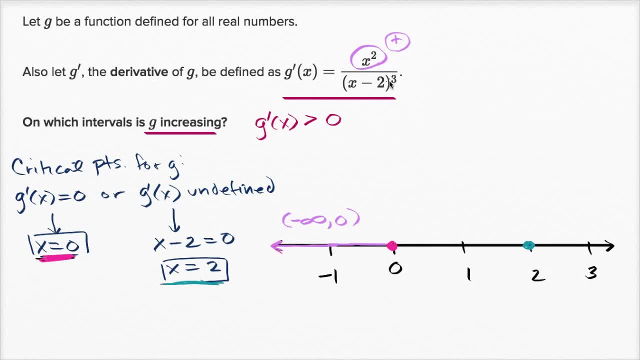 you're still gonna get a negative number and then you take it to the third power. Well, a negative number to the third power is gonna be a negative number, So that right over there is going to be negative. So you're gonna have a positive divided by a negative. 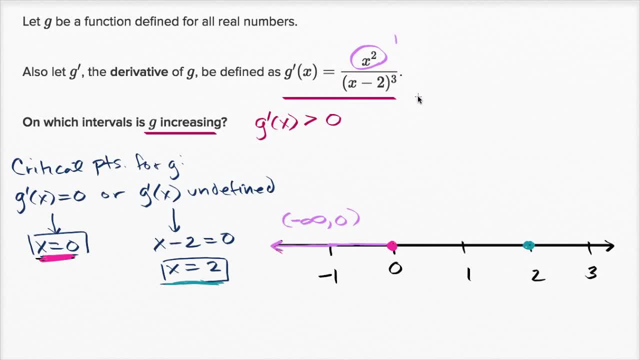 So g prime is going to be negative, So let me write that down. So, on this interval, on this interval, I'll write it like this: g prime of x is less than zero, or if we cared, or if we wanted to know when it's decreasing. 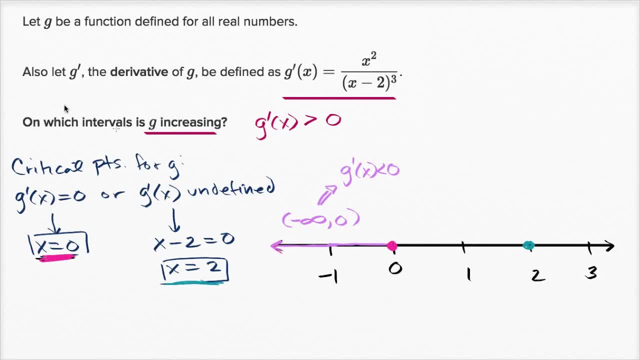 we would know it's definitely decreasing over that interval. Now let's take. let's take the interval between between zero and two Right over here. So this is the interval from zero to two, the open interval. So what's gonna go on with g prime of x here? 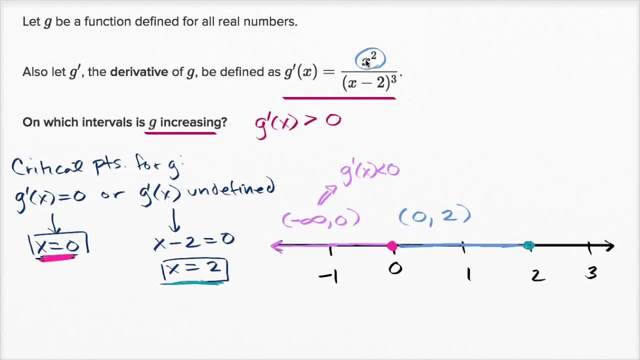 Well, once again, x squared anything greater than zero, and it says we're not including zero in this interval. well, this is for sure going to be positive. And so let's see if we have x minus two, where x is greater than zero. 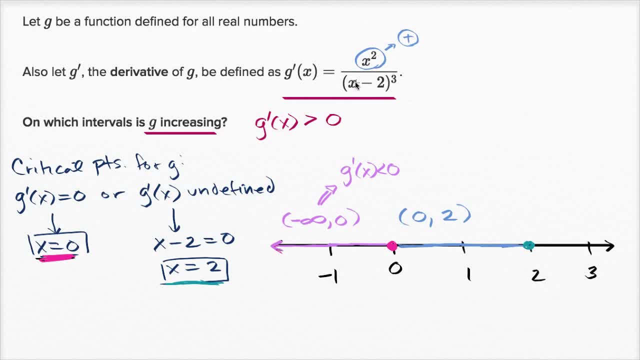 but less than two. so if x, we could just say, for example, if x was one, one minus two is negative one. We're still gonna get negative values in this denominator right over here. So, since we're still gonna get negative values, 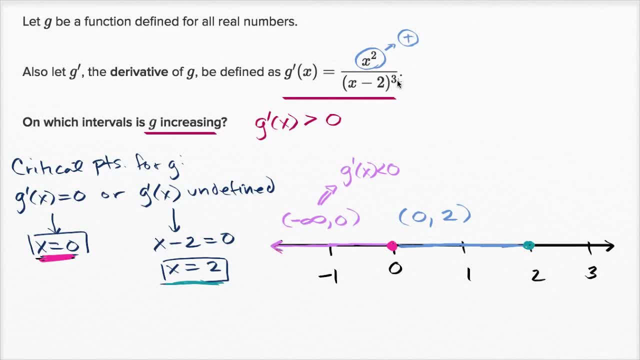 in this denominator. the denominator is still going to be. take a negative value to the third power. well, you're gonna still get a negative value. So this is going to be negative. So you're still going to have g prime as less than zero. 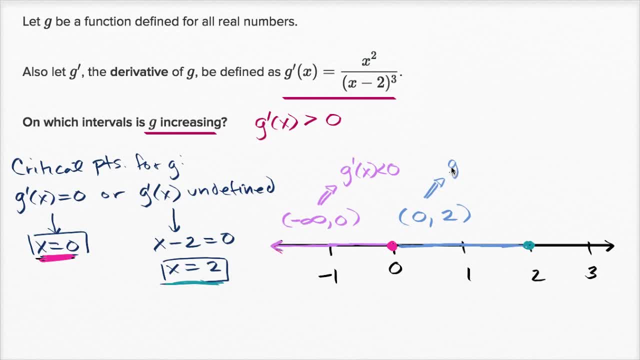 So let me write that down. So you still have g prime of x. g prime of x is less than zero. And then let's take the interval above, Let's take the interval from two to infinity. Two to infinity. Well, the numerator is positive. 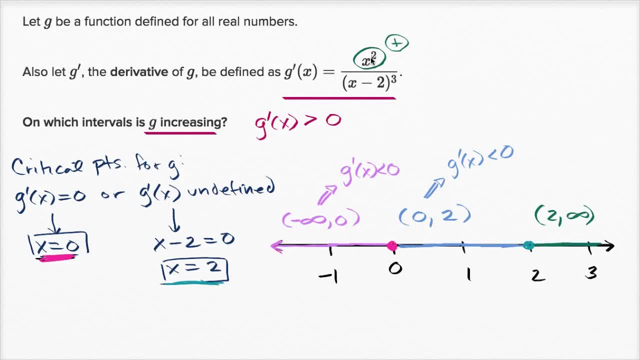 it's always gonna be positive for any x not being equal to zero And this denominator. you're taking values greater than two, subtracting two from it, which is still gonna give you a positive value. You take the third power: it's all gonna be positive. 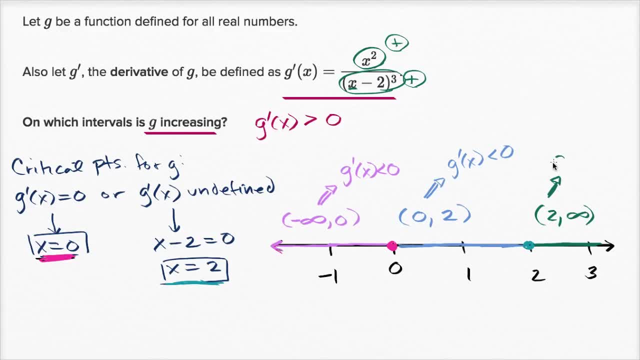 It is all going to be positive. So this is the interval where g prime of x is greater than zero. So on which intervals is g increasing? Well, that's where g prime of x is greater than zero. So it's going to be from two. 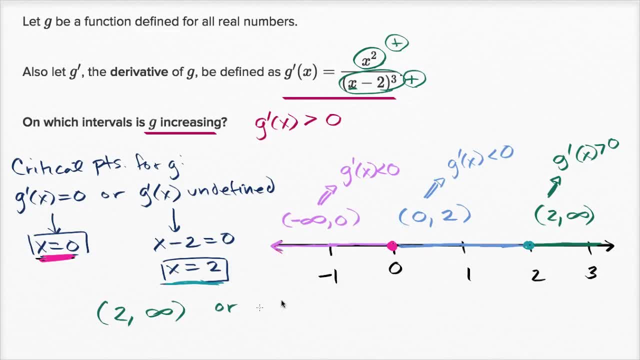 from two to infinity. Or we could just write it like this: We could write: x is greater than two. Either way, for either of these, g prime of x is greater than zero and your function, g is zero, Is going to be increasing.